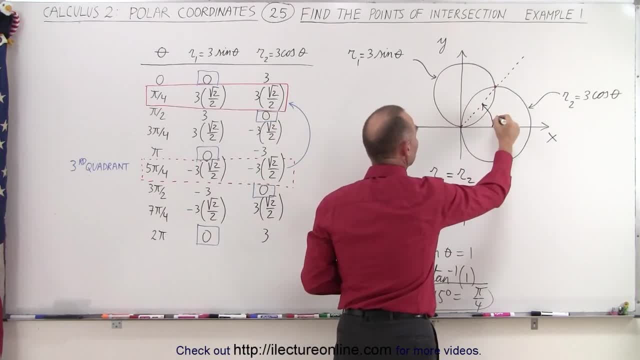 and you can see that when we graph it, that's obviously the case at an angle of 45 degrees. and you can see that when we graph it, that's obviously the case at an angle of 45 degrees. so when we take this angle here and we realize this angle, theta equals 45 degrees, which is pi over four. 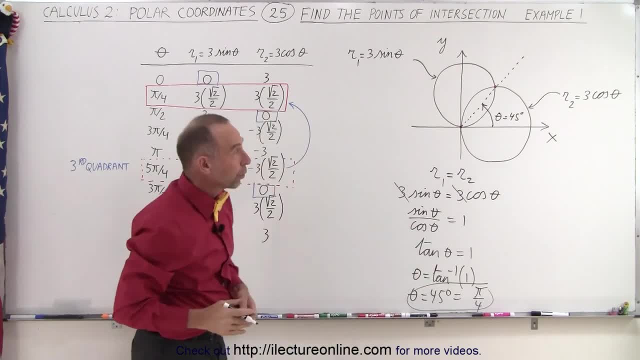 then you can see that that's where they're going to meet, that's where they're going to overlap, that's where there's going to be a point of intersection. But somehow we missed a point. We can see graphically. there's another point of intersection at the origin, when R is equal to zero. 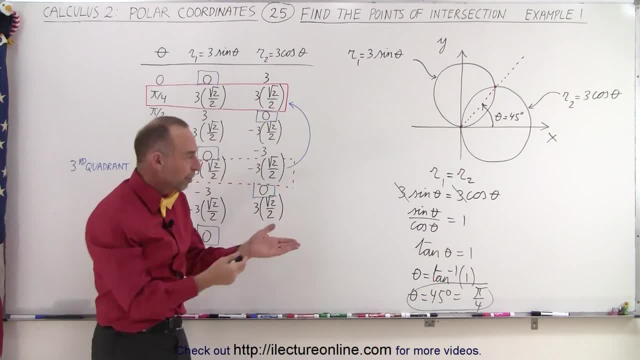 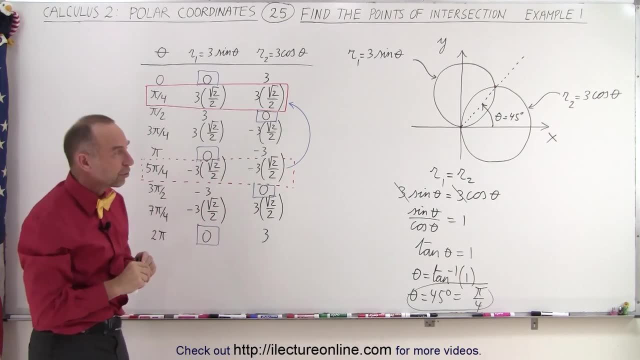 but we didn't find that using the method of setting the two equations equal to each other, but we didn't find that using the method of setting the two equations equal to each other. So here, if we take a look at this, and we're going to take another look at the graph- 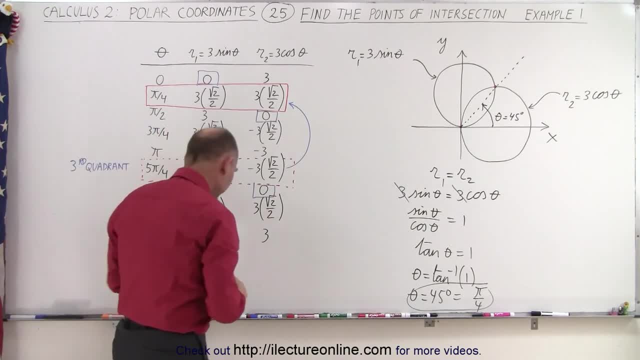 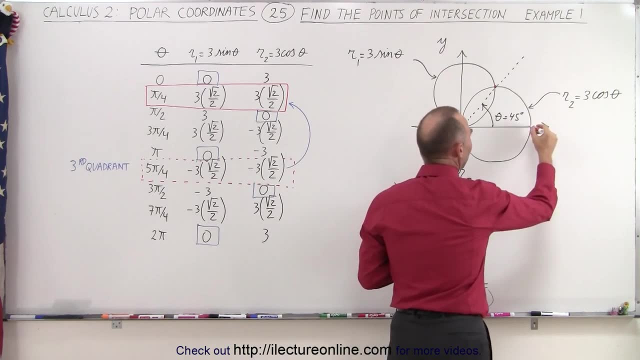 you'll see there's a reason why that was the case. For example, notice that when the angle is zero degrees, that gives us a point right here on the graph for R2.. So this is the point where theta is equal to zero for R2,. 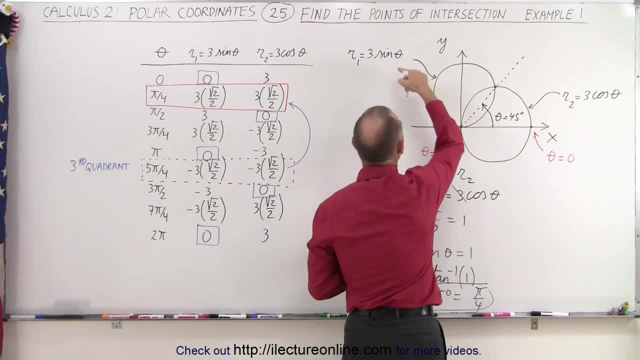 but this is the point where theta is equal to zero for R1.. So, in other words, when R1 equals zero, R2 equals zero. R1 is at the origin. R2 is out here on the x-axis, a distance away from the origin. 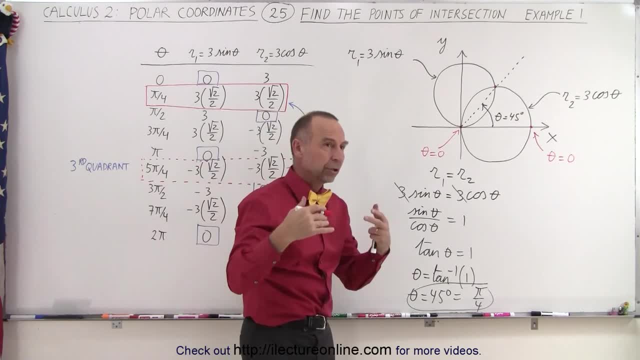 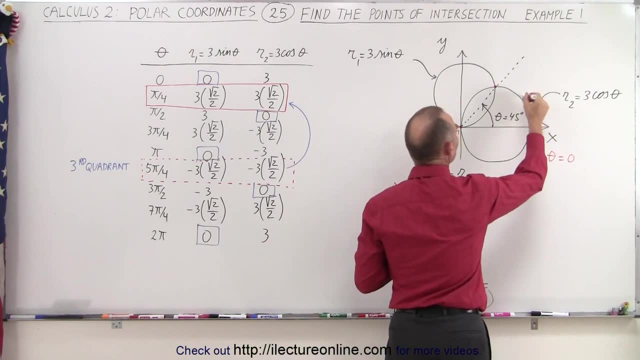 so they don't occur at the same time. After we let theta go another 45 degrees- notice 45 degrees in this direction, along this curve, puts it at this location, and the same 45 degrees along this curve gets us at the same location. 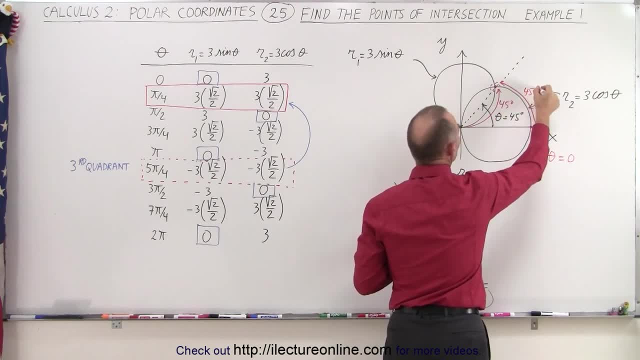 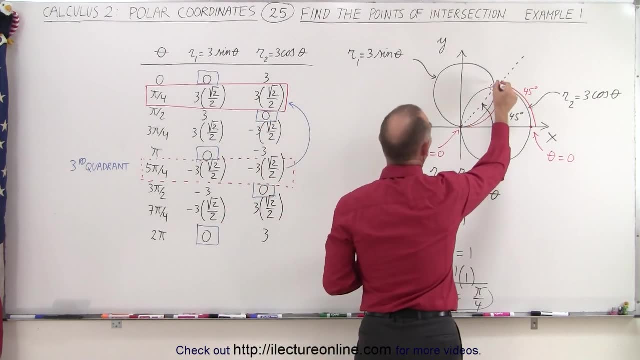 So when theta is 45 degrees, and 45 degrees here, notice, we end up at the same point, and that's the point that we found. Then if we go another 45 degrees, notice at this point, another 45 degrees. the cosine function then reaches the origin. 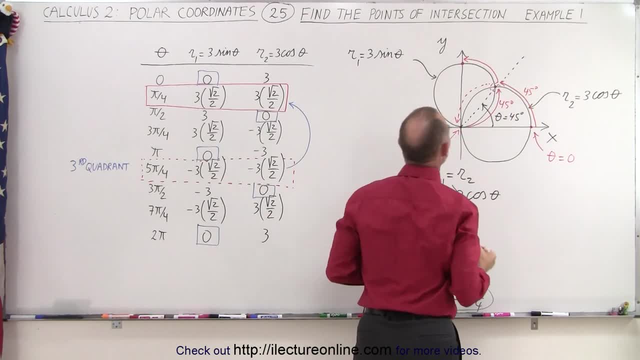 but if I go another 45 degrees along this curve right here, I end up at this location. So at the very beginning, when the angle is zero degrees, the sine function was at the origin. but the cosine function doesn't reach zero degrees until the angle has reached 90 degrees. 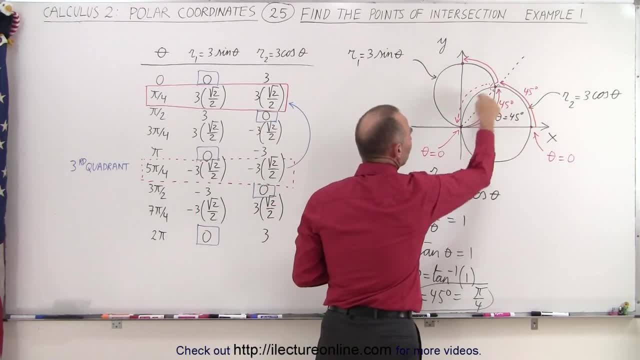 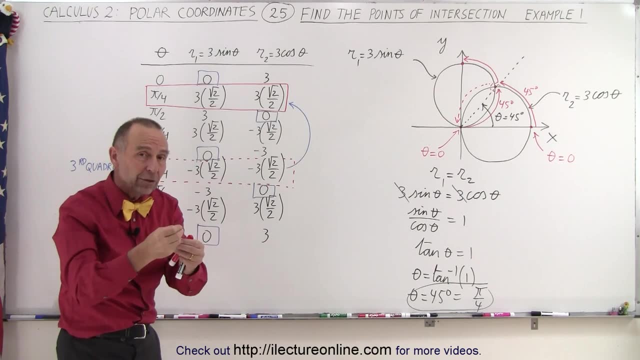 Or I shouldn't say, I should say, I should say that the cosine function doesn't reach origin until the angle is 90 degrees. So that means that they do both get at that location, but not for the same angle, theta. So there is an intersection. 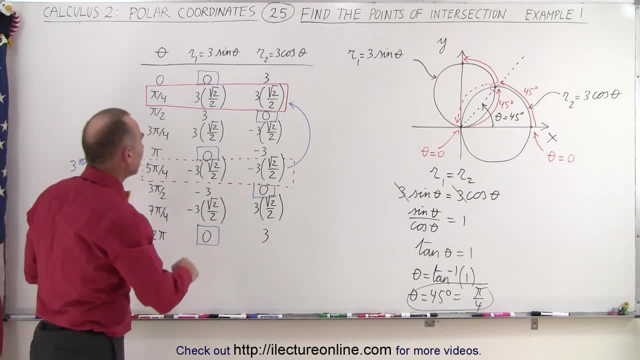 it just doesn't occur when theta is a particular value. You can see that here the first function reaches zero, there the second function, the first function, the second function, the first function, so forth. So they do overlap, just not for the same angle: theta. 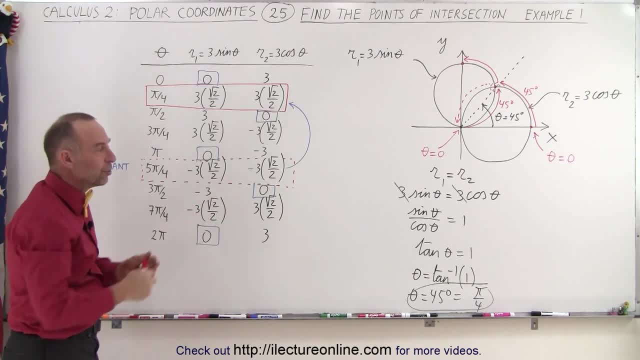 So we need to recognize that there's a point of intersection. you just can't find it using this technique. Now, what about this point right here? Because if I take a look here, notice when the angle is 5 pi over 4,. 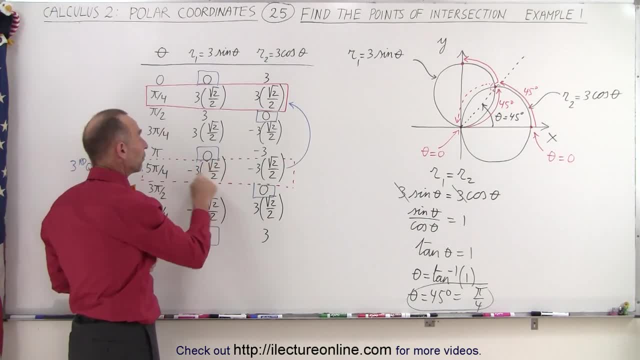 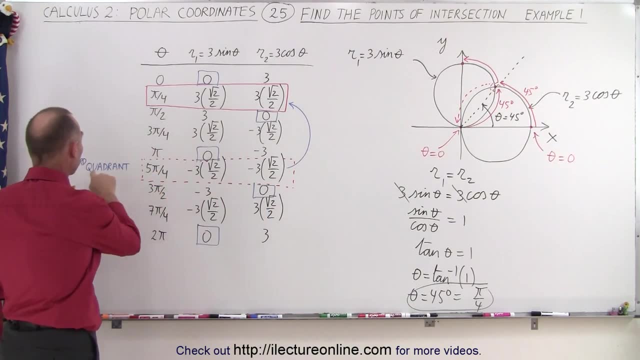 they both have the same value, minus 3 times the square root of 2 over 2.. So why would that not be a third point of intersection? Well, it turns out that this is at the third quadrant, and in the third quadrant both the sine function and the cosine function have negative values. 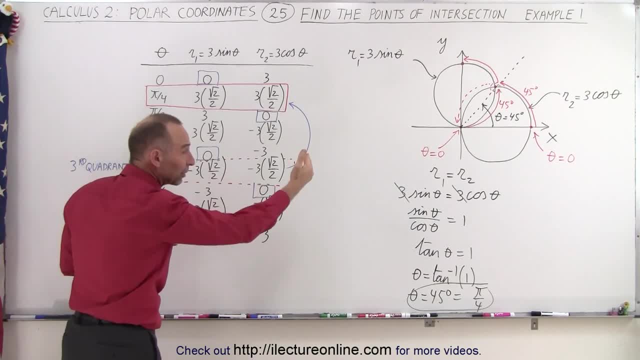 So if you multiply these both by a negative value to get the r value, the distance away from the origin according to polar coordinates, they'll put you back at this location right here. So what we can do here is take a look. 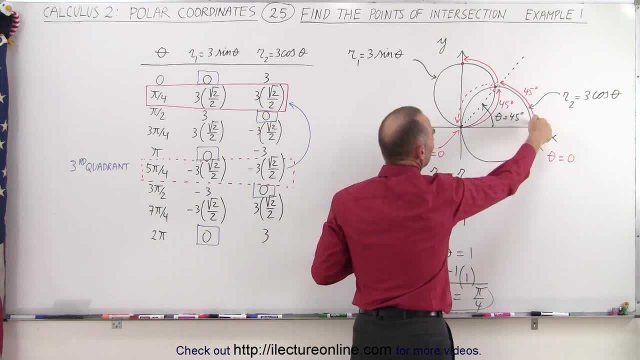 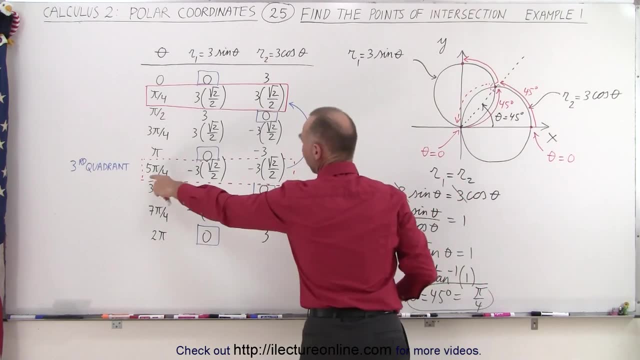 So we go 90 degrees, 180 degrees, which is pi. then we go another pi over 4 here. now we're back at this location, same over here, If we travel a complete distance of 5 pi over 4,. 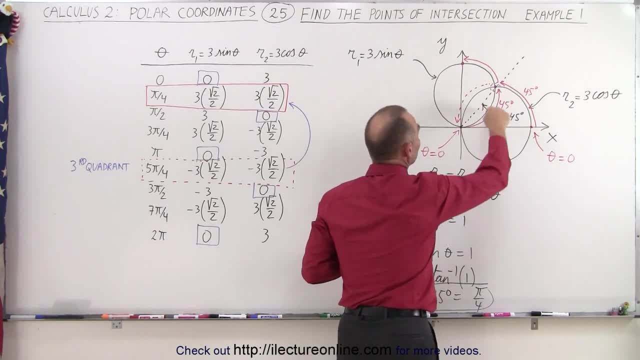 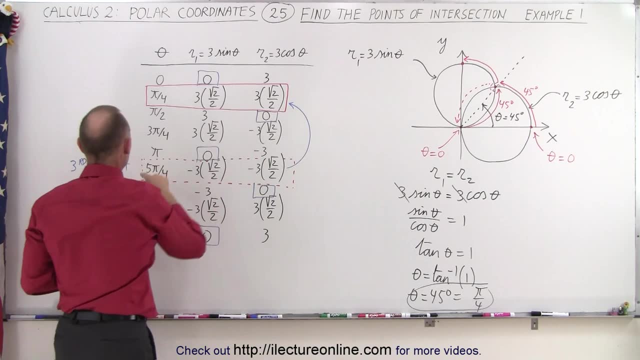 angular distance, that is, according to the value theta notice, then we get back at this location. So even though, according to the values we would get if we plug in bigger and bigger angles and eventually the angle 5 pi over 4, we get these two values being negative. 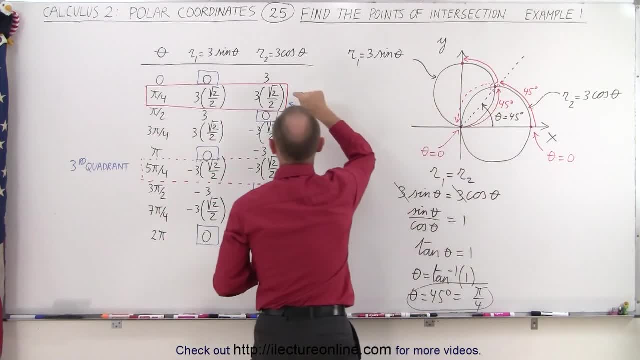 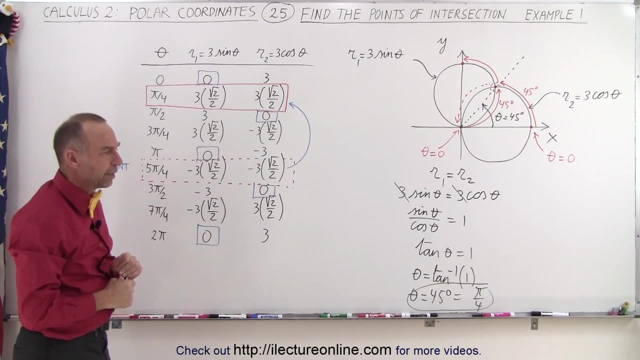 it puts us back at this location, right here, the same point that we found before at this location. So there really isn't a third point of intersection which you might assume by looking at this value. So that's why I say it is a bit tricky. 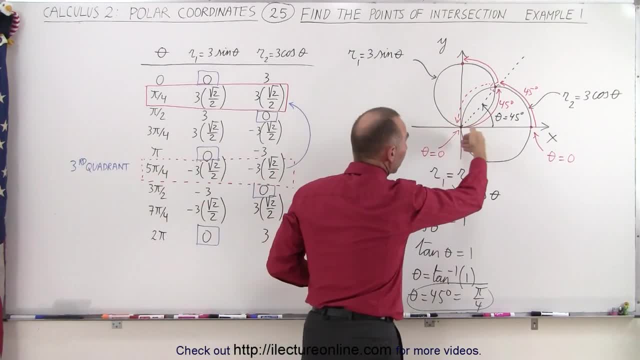 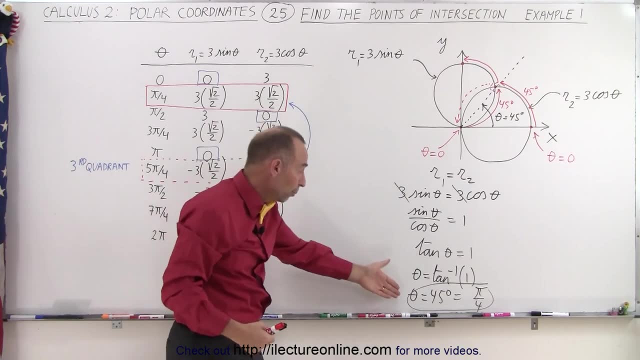 What you should do is first of all graph the functions, which gives you a visual picture of where the points of intersection may be. Then work it out like this, like you would traditionally, which probably will give you at least one of the points of intersection.